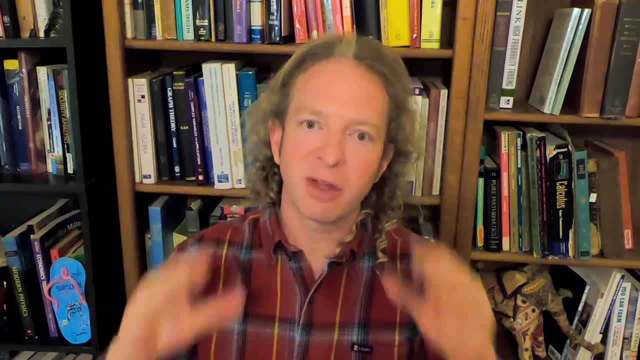 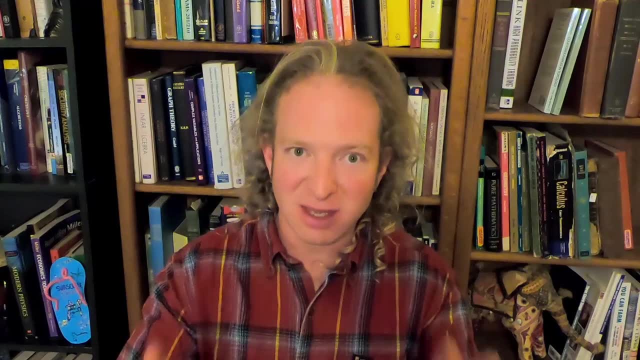 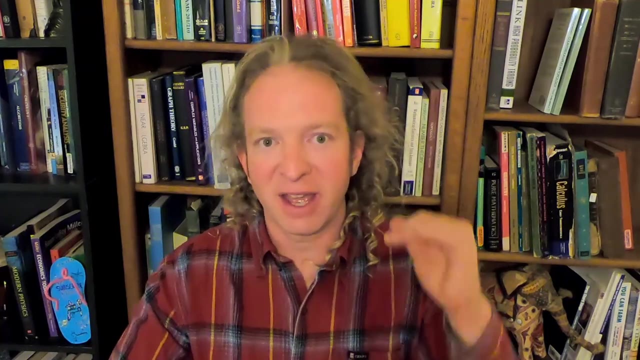 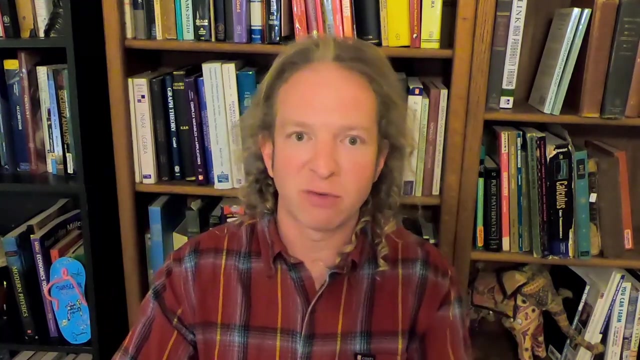 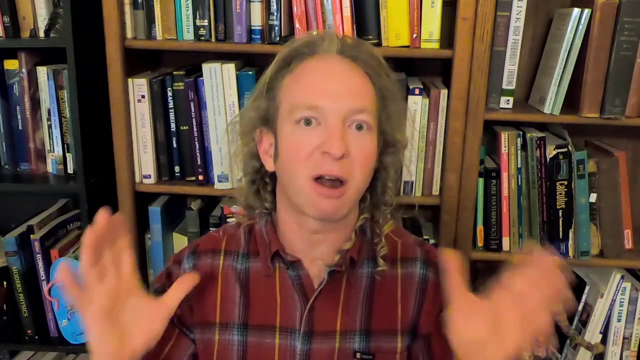 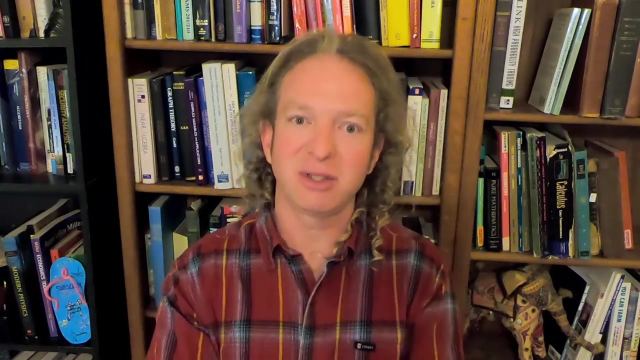 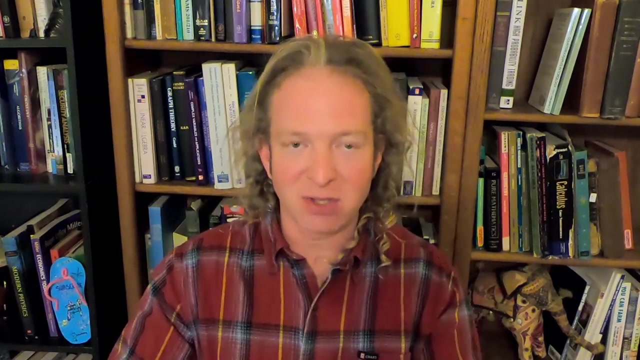 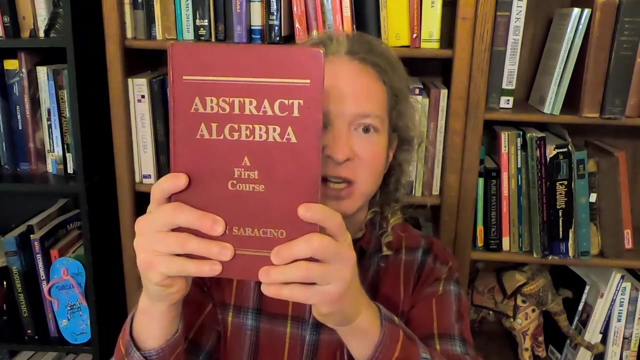 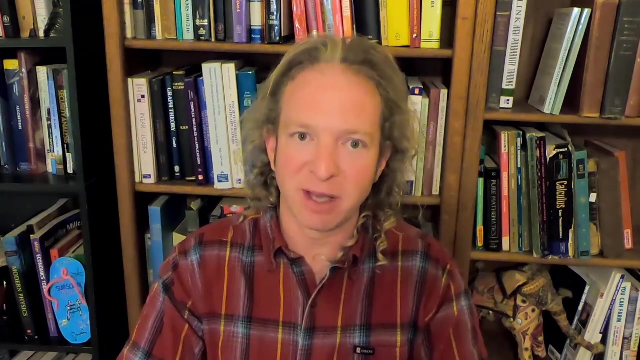 Hey everyone, in this video I want to go over four books that are awesome for beginners in abstract algebra. So if you're trying to learn abstract algebra, I think these might be the four best books that you can get on abstract algebra. Now first let me just say that I have in-depth reviews on these books. I've done in-depth reviews on these books and I'll leave the links to the books and reviews in the description. But in this video I want to just talk briefly about all four of these books because these books are amazing. I have over 25 abstract algebra books and I think these are the best ones for beginners. Some of them are a little more advanced but let's get started right away. So the first book that is extremely good for beginners is this one right here. Abstract Algebra by Dan Saracino. The Saracino book is absolutely beautiful. This in my opinion is the absolute best book for beginners. 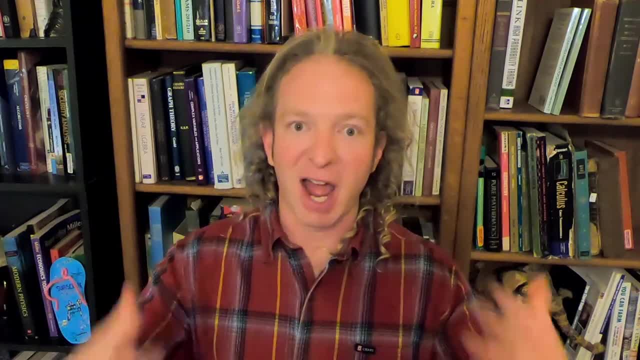 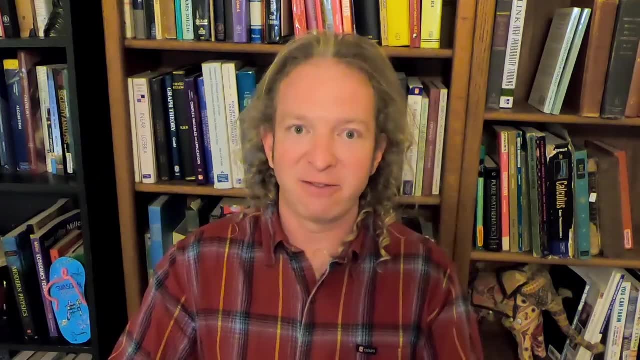 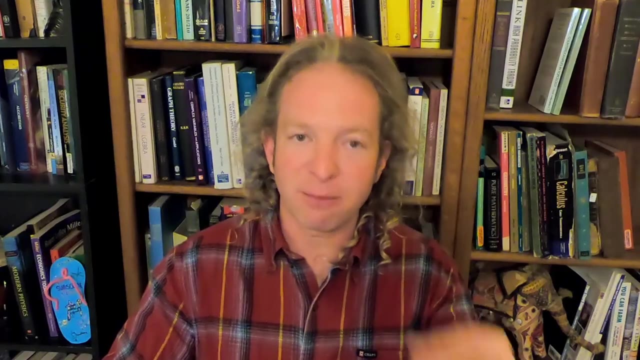 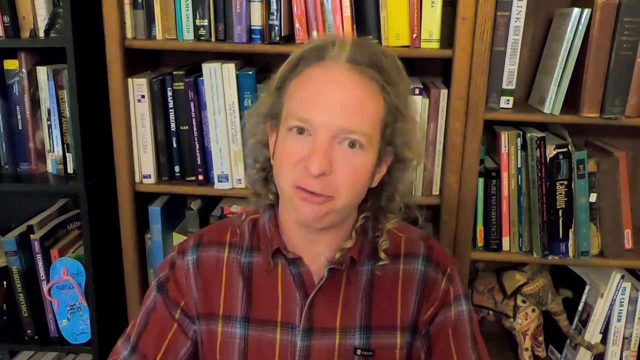 Now I am a little bit biased. This is the book that I used when I took abstract algebra. I had also an amazing professor so I was very very lucky and very very fortunate. I have read this entire book. Sometimes people ask me, do you actually read all the math books you do reviews on? Absolutely not. But this book here, I have read the entire book and I have done almost every single 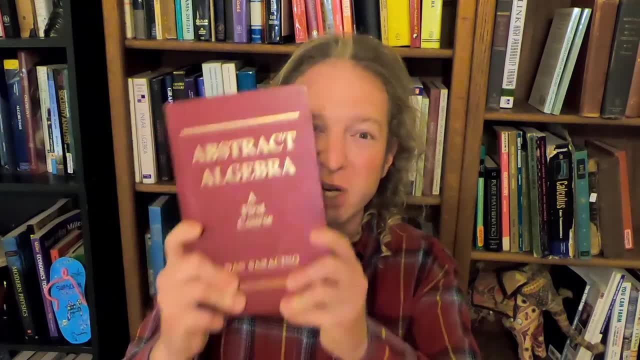 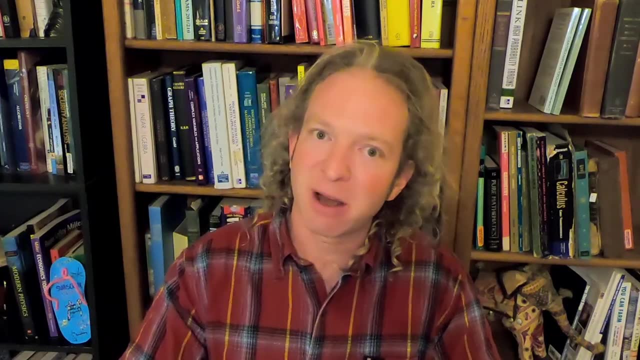 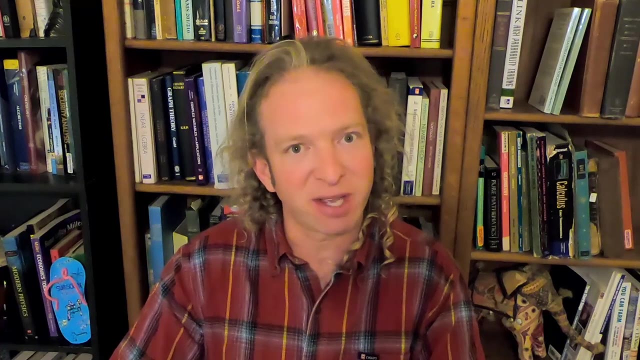 problem. I did find the book lacking. It does not have everything. It talks a little bit about UFDs and PIDs but it doesn't go into much more. It doesn't mention group actions and stuff like that. It doesn't mention semi-direct products. So again, it's a good beginner book. So number one book, 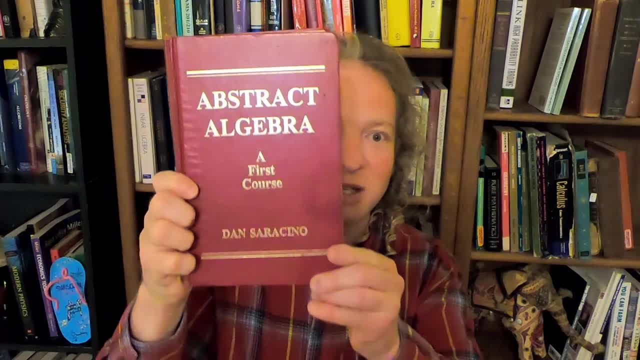 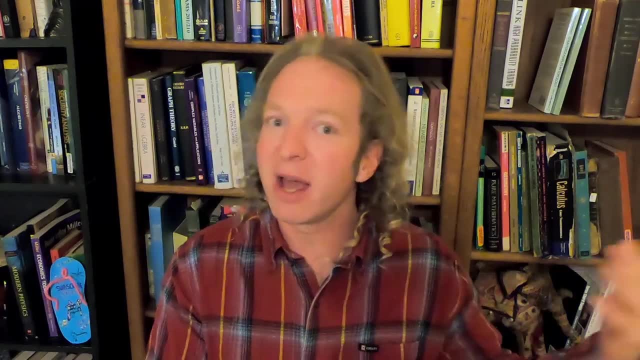 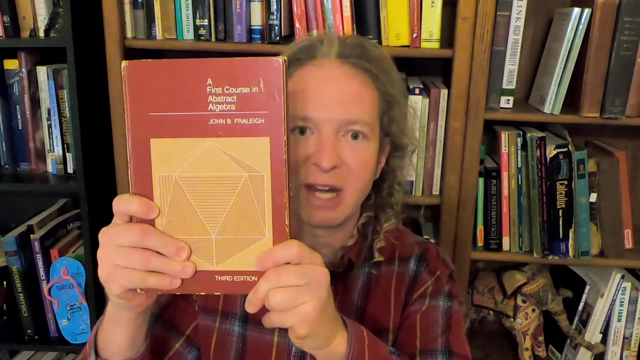 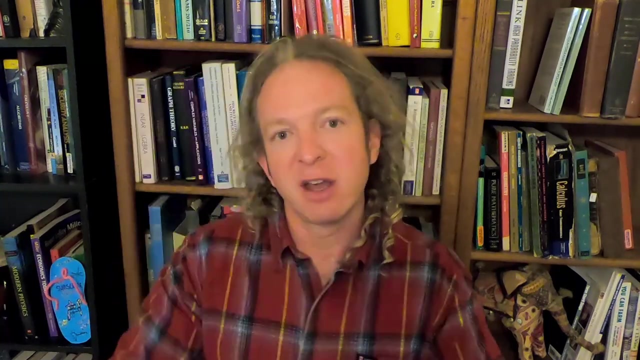 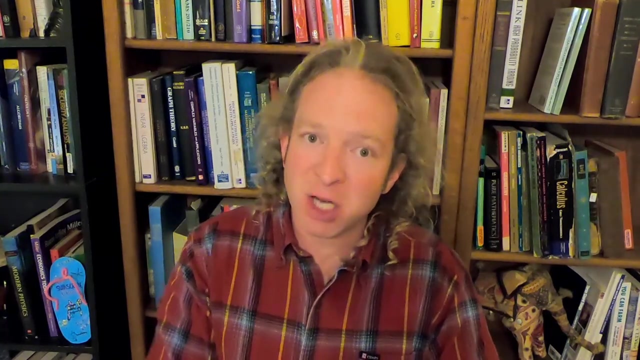 Abstract Algebra, a first course by Dan Saracino. That is a must have if you are learning abstract algebra. And again, it's the best beginner book in my opinion. Why? Because I used it and I am biased. But I do love the way it reads. It is a very very gentle introduction. This is the second book that I would recommend. This is a first course in abstract algebra by John B. Frillet. This is the Frillet book. This book was recommended to me by my abstract algebra professor when I took the course many years ago. This book has much more information than the Saracino book. Here it is again so you can see it. 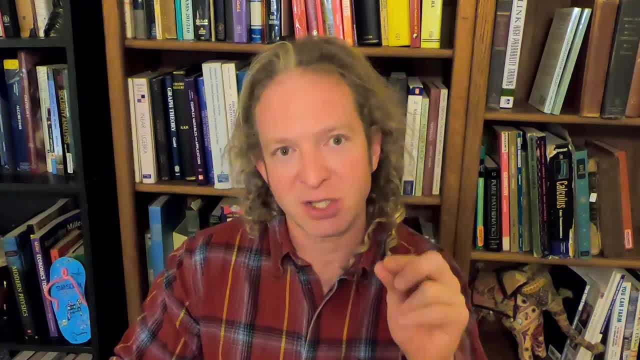 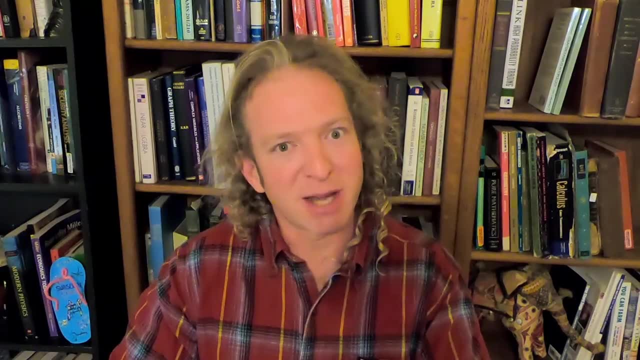 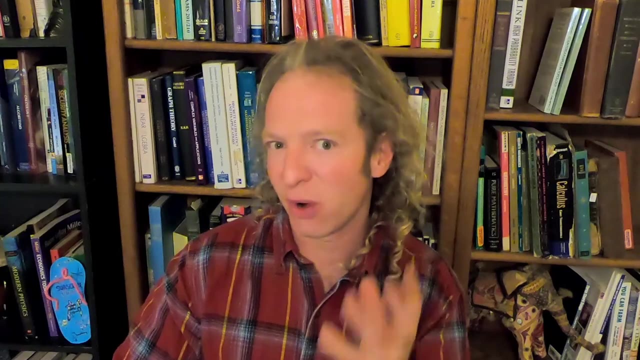 It's much more in depth. The Frillet book has really small sections similar to the Saracino book but it has many more sections. Downsides of this book, it's a really minor thing but the way the author does the multiplication of the cycles, he does it in a very non-standard way. 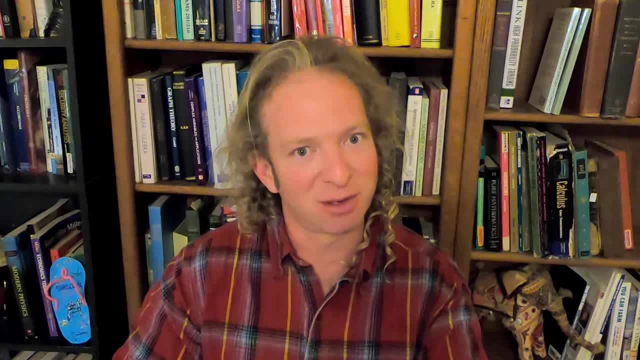 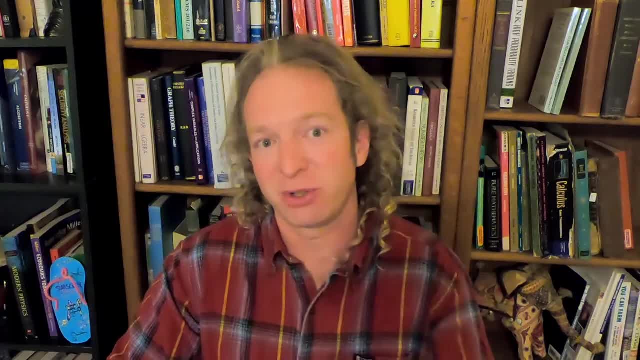 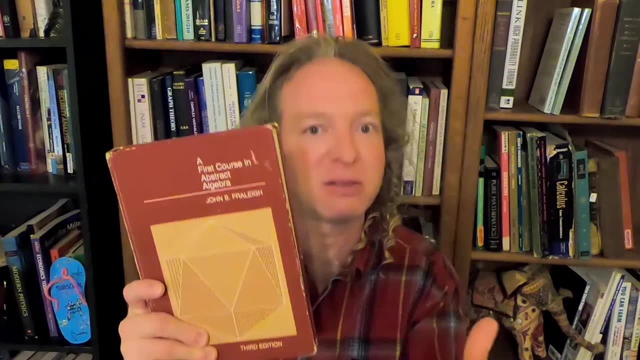 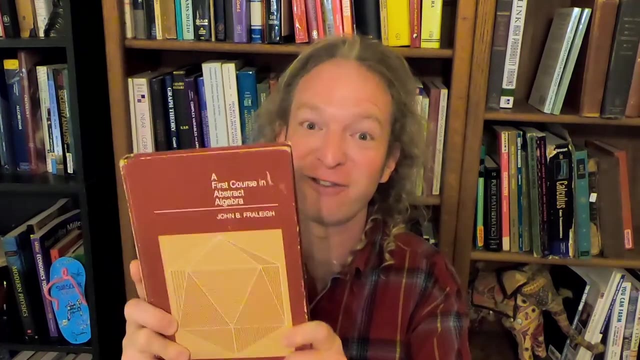 It's a really good read. This book also has a really good introduction. It talks a little bit about definitions in mathematics, how mathematics works. It's a beautiful book. Again, this is the Frillet book. I love this book. I have read also most of this book. This is the third book that I 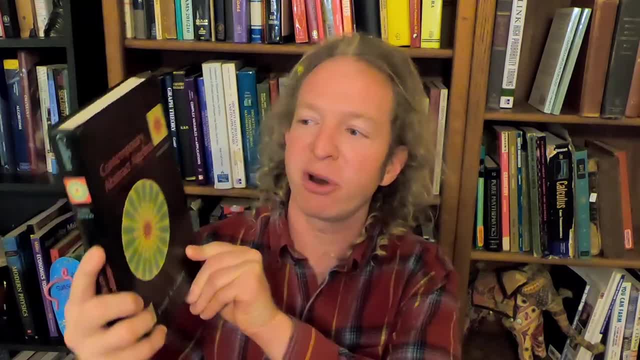 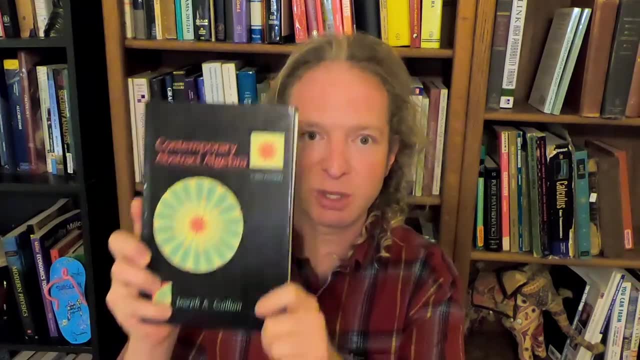 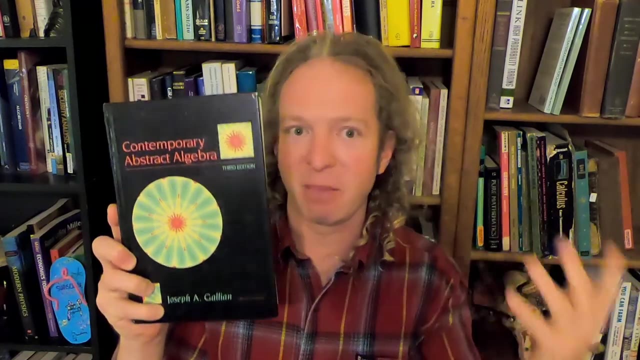 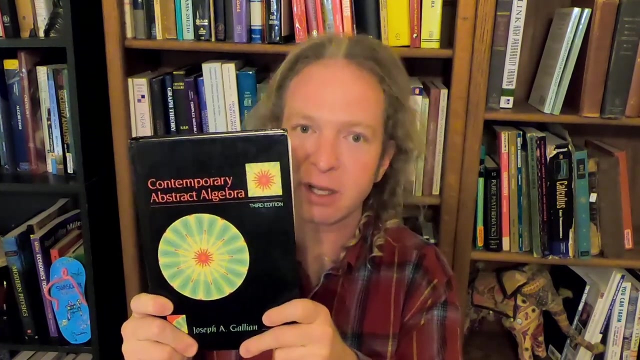 wanted to discuss. This is the book by Galleon. It's called Contemporary Abstract Algebra. My really good friend from New Zealand who has his book, Contemporary Abstract Algebra, he's going to who has his PhD in mathematics, he used this book for a course he took at the University of Auckland. He loved the book so I bought it and I love the book. I use this book mainly as a reference and as a source for examples. I have done some of the problems from the book and I 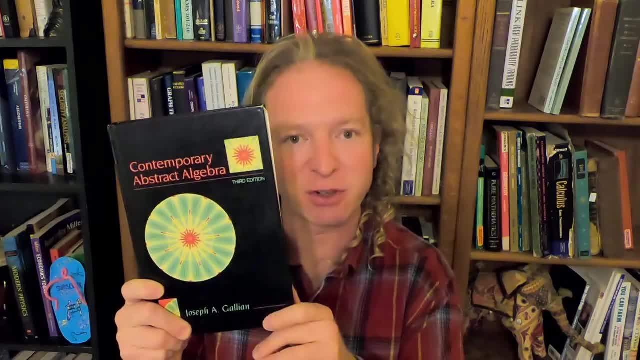 have read some of the sections, in particular the sections on rings and factor rings, but 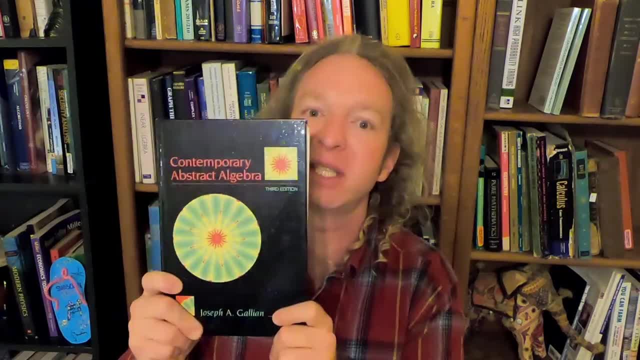 mainly as a reference. This is a book of examples. When I think of the Galleon book, I think of a book of examples. When I think of the Galleon book, I think of a book of examples. 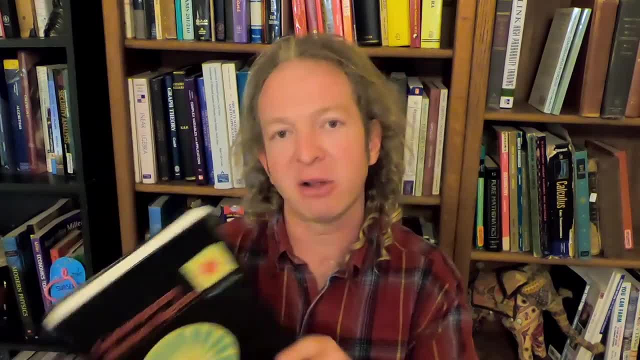 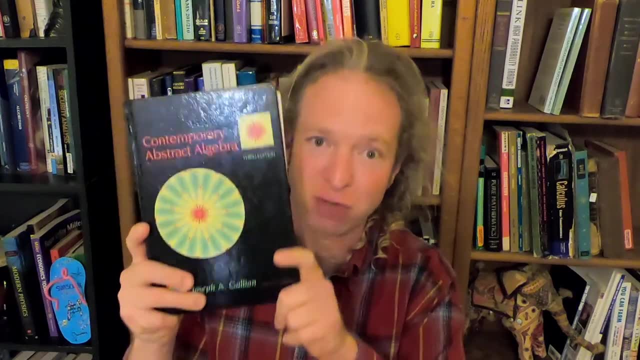 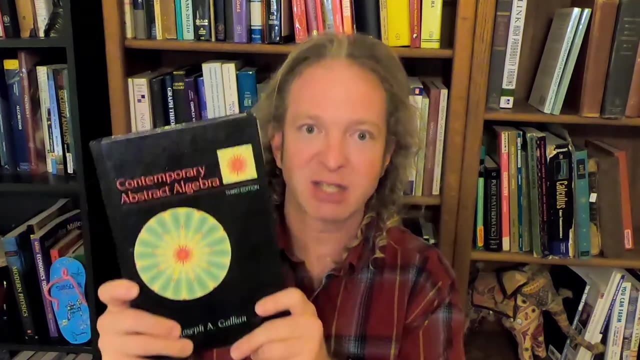 I've done a review on this book and again, I'll leave a link to the review and the book in the description. Many people have used this book in their courses and they have been extremely happy with this book. I think this is a solid book. My friend loved this book. I like the book. Again, it's the Galleon book. Excellent choice for beginners in abstract algebra. 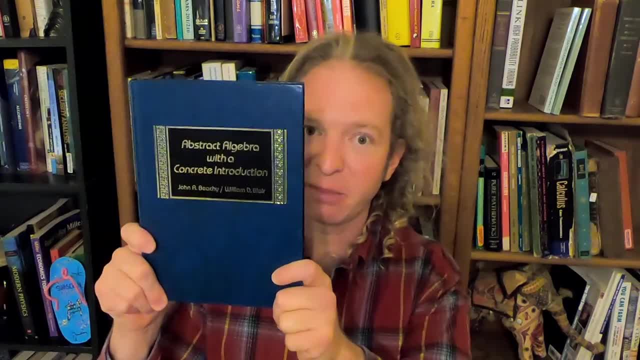 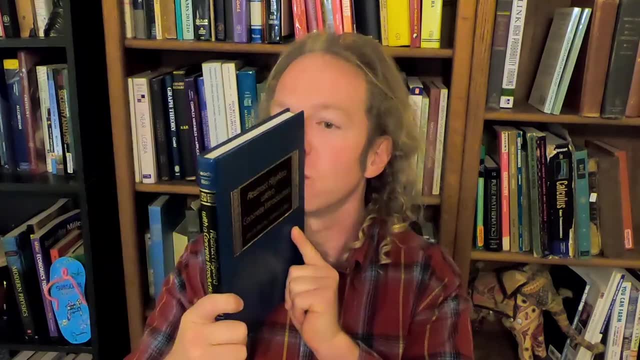 This is the third book that I would recommend. This is the Beachy and Blair book. I found this book on Amazon via Google many years ago. I did some research and I bought the book. My copy is brand new. This is a new edition or a new copy rather. Abstract Algebra with a Concrete